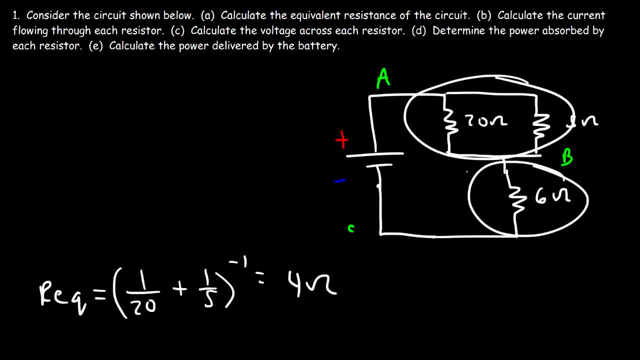 resistor of 4 ohms, which is going to be in series with a 6 ohm resistor. So therefore the total resistance of the whole circuit is going to be 6 plus 4, which is 10 ohms. Now I'm going to redraw the circuit on the right side so I have more space to put other 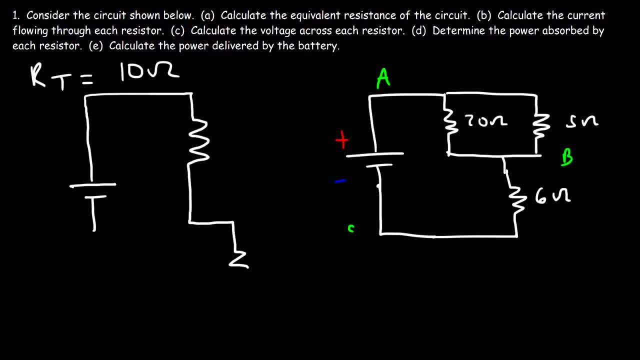 stuff. So this is 20 ohms, this is 5 ohms and this is 6 ohms, and the voltage of the battery is 20 volts. So this is 20 ohms, this is 5 ohms and this is 6 ohms. 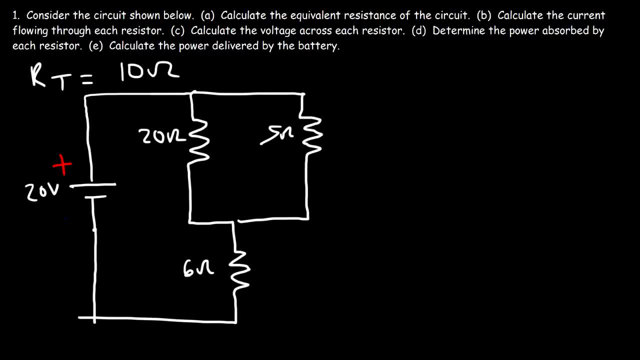 Now, what do you think we need to do next at this point, Now that we have the equivalent resistance? With this information, we can calculate the total current that flows in a circuit. So it's going to be the voltage of the battery which is equal to the current in the circuit. 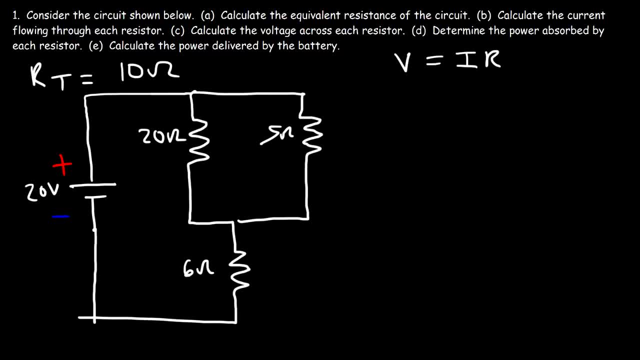 times the resistance. V equals, I R Ohm's law, So the total current In the circuit it's going to be the voltage of the battery divided by the total resistance. So it's 20 volts divided by 10 ohms. 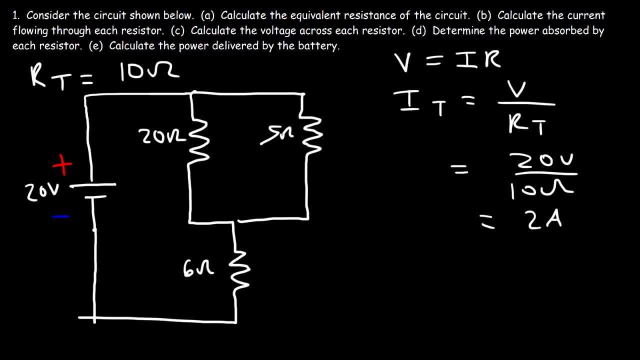 So there's a total current of 2 amps flowing in the circuit. So that's how much current leaves the battery. It's 2 amps, Which means that 2 amps of current must also enter the battery, which means 2 amps of current. 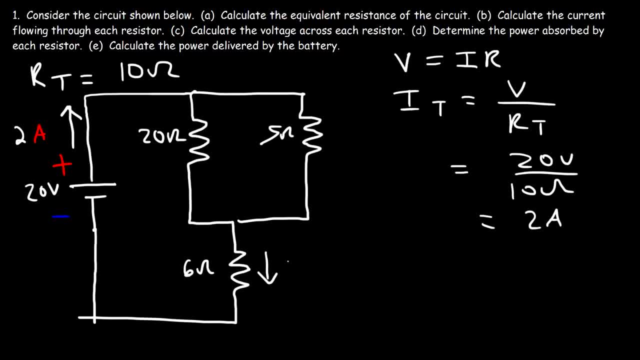 flows in this direction. So there's 2 amps of current That flows through this resistance. Now the total current that flows in these two resistors has to be 2 amps. but we'll get there. We'll talk about how to figure it out. 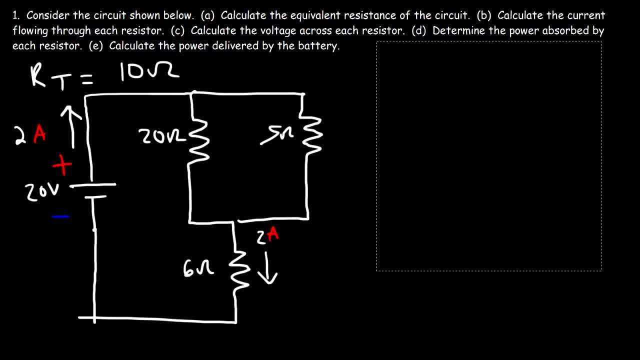 Now here's a question for you. Will there be more current flowing through the 5 ohm resistor or through the 20 ohm resistor? What would you say? If you decrease the resistance, the current will increase. So what would you say? 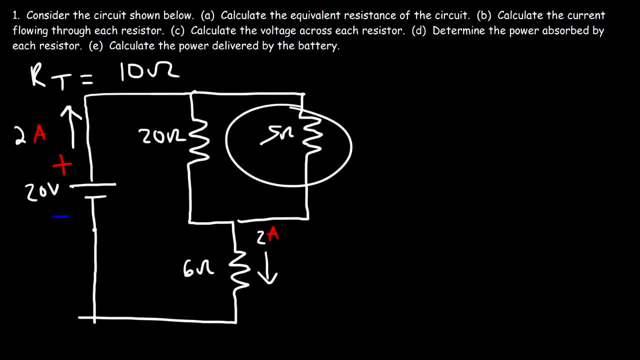 If you decrease the resistance, the current will increase. So there's going to be more current that flows through this resistor Now, because 20 is 5 times the value of. I mean it's 4 times the value of 5, we should. 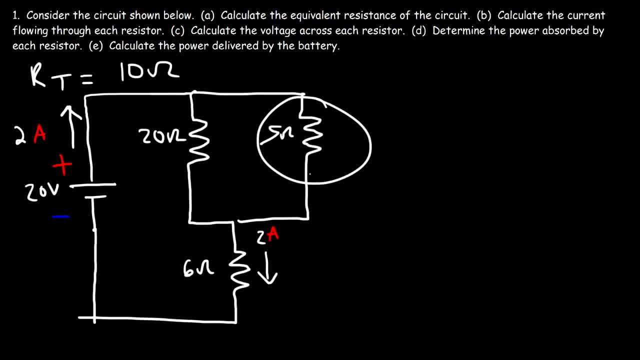 expect that the current that flows through the 5 ohm resistor should be 4 times as great compared to the current that flows through the 20 ohm resistor. Now the total current has to be 2 amps, So how can we use this current to figure out what the currents are in these two resistors? 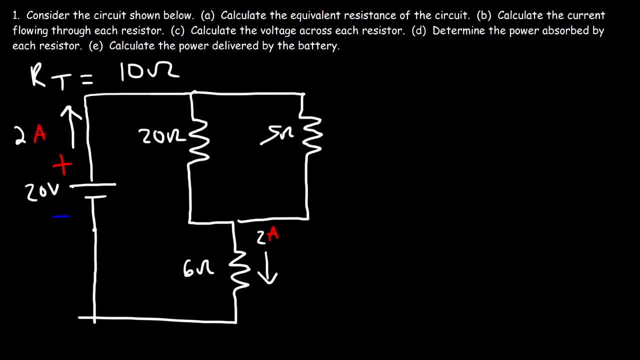 There's two ways in which we can find the answer. Now here's a formula that you can use. So if you want to find, let's say we'll call this R1 and R2.. Let's say, if you want to find the current in R1, and you know the total current in these, 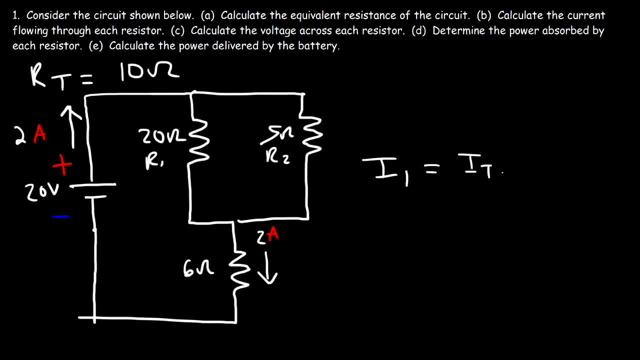 two branches. it's going to be the total current times, the other resistor, R2, divided by the total resistance, R1 plus R2.. So the total resistance is 20 plus 5, which is 25.. And the other resistor is 5.. 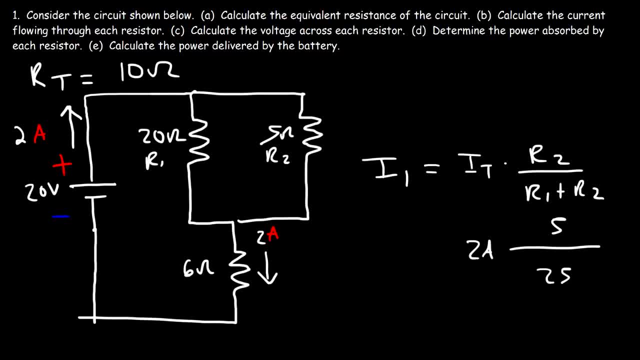 The total current in those two branches is 2 amps, So 5 out of 25 is 1 fifth. so it's 1 fifth of 4, I mean 1 fifth of 2.. So therefore, there's only 0.4 amps of current flowing through this resistor. 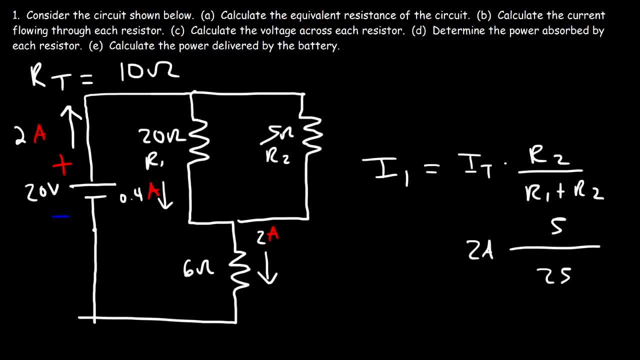 So the total current in these two branches is 2 amps. So 5 out of 25 is 1 fifth. so it's 1 fifth of 2.. Now to calculate I2, you can use this formula: It's going to be the total current, which is 2 amps, but it's going to be R1, the other. 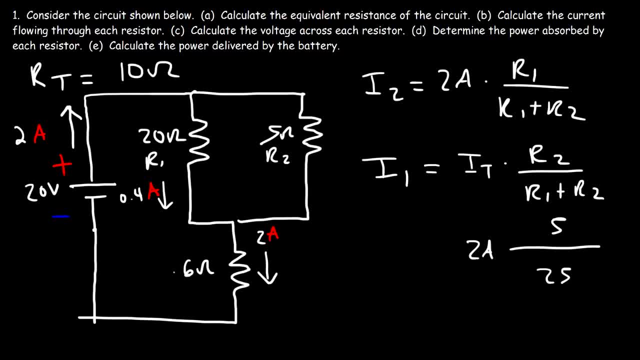 resistor over R1 plus R2.. So R1 is 20 ohms and the total resistance is 20 plus 5, or 25.. So it's 2 times 20 over 25.. And so the other 1.6 amps flows in this form. 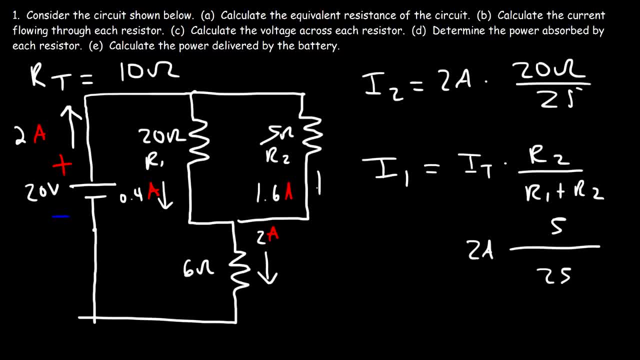 And, as you can see, the total current 0.4 plus 1.6, adds up to 2.. So now we have the current flowing through each branch. Now it turns out that there is another way in which we can get the same answer. 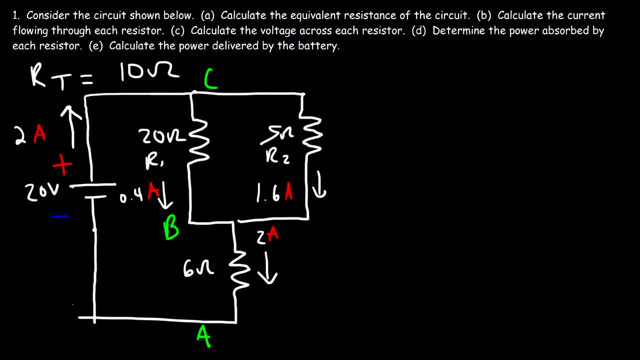 Let's call this point A, B and C. You need to know that the voltage Between points A and B, that is, across the 6 ohm resistor, plus the voltage between points B and C, which is the voltage across R1, and that's the same as the voltage across R2, because 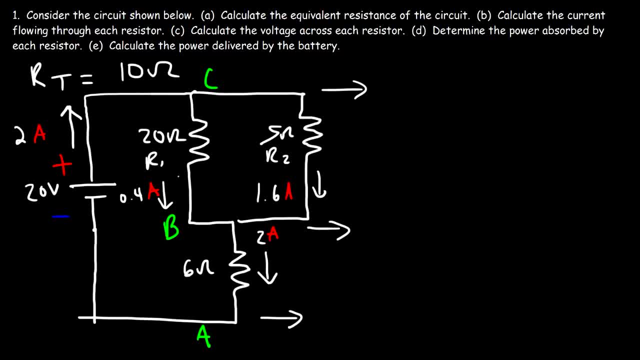 those two resistors are in parallel, The sum of these two voltages have to add up to 20.. Now we can calculate the voltage between points A and B, because we have the current flowing through the 6 ohm resistor. So V equals IR. 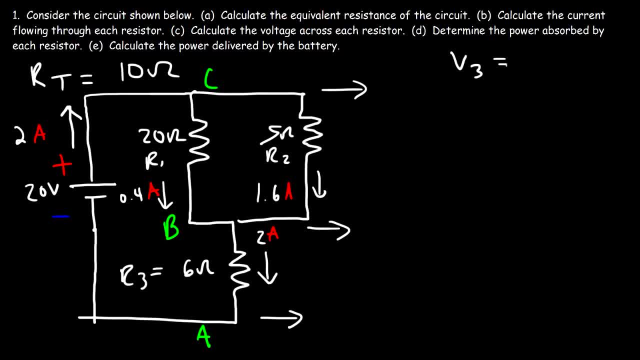 Let's call this R3. So the voltage across R3 is the current that flows through it times R3. So the current that flows through it is 2 amps. R3 is 6 ohms, So the voltage across R3 is 12 volts. 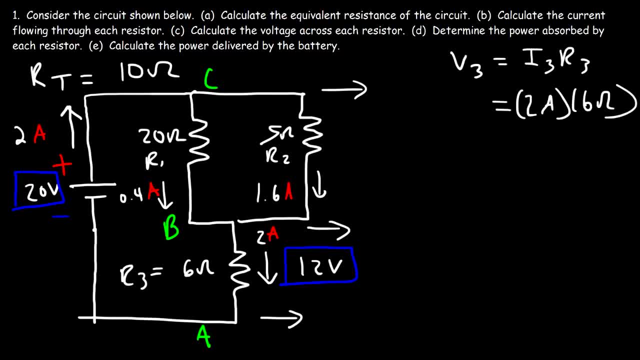 Now 20 minus 12 is 8.. So the voltage across R1 and R2 has to be 8 volts. So now we can calculate the current in R1 and R2. and R2.. So the current is going to be the voltage across R1 divided by the resistance of R1.. So the 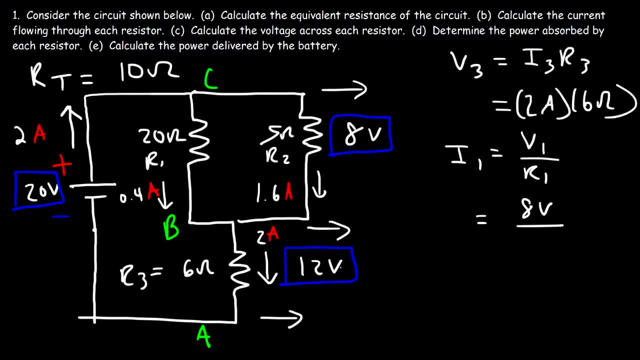 voltage is 8 volts and the resistance is 20.. So 8 divided by 20 will give us 0.4 amps. Now for the other one, I2. it's going to be the voltage V2, which is also 8 volts, divided by R2.. So that's going to. 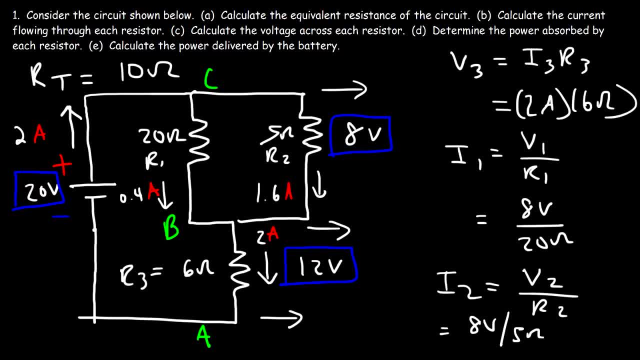 be 8 volts divided by 5 ohms. If you take 8 and divide it by 5, that will give you 1.6.. So that's another way in which you can calculate the current flowing in those branches. Now let's determine the.